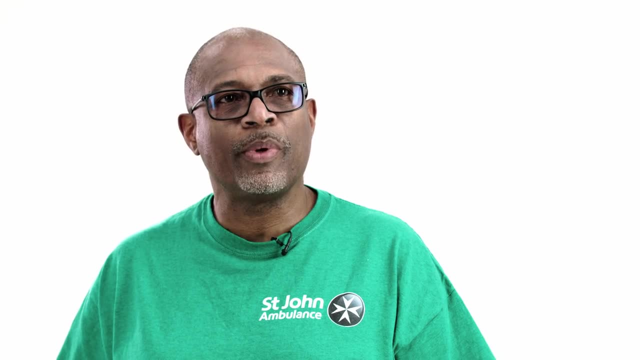 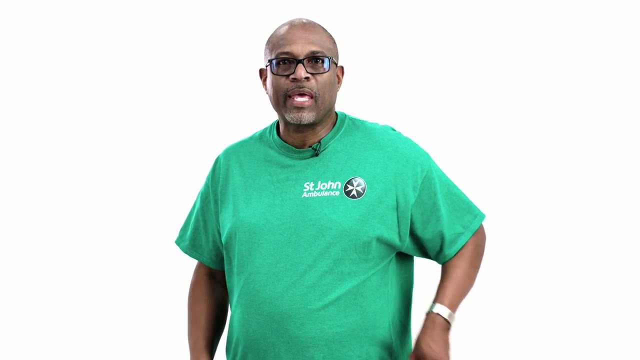 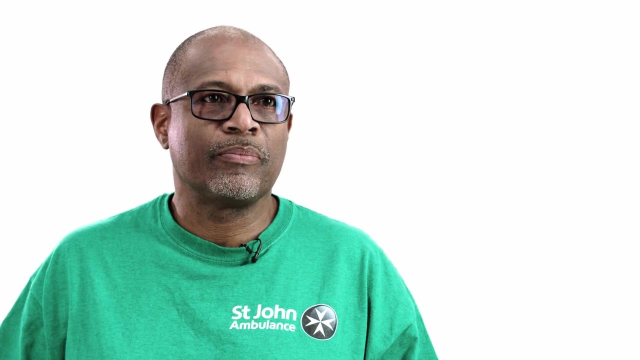 their lips, the earlobes or the nail beds. People with asthma usually know how to deal with their own attacks by using their liver inhaler, usually with a blue cap, at the first sign of the attack, But if they don't, or if the attack is severe, you may need to help. 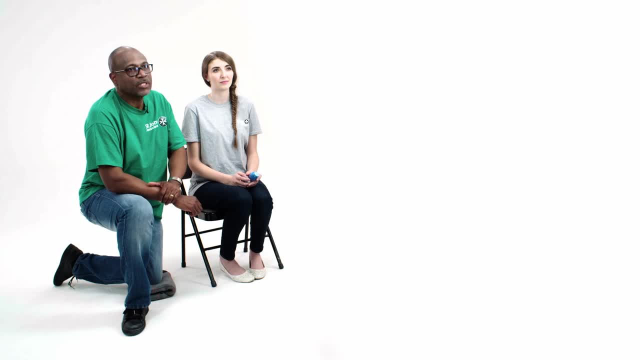 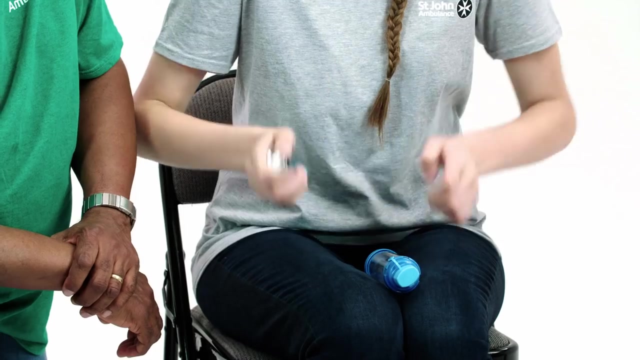 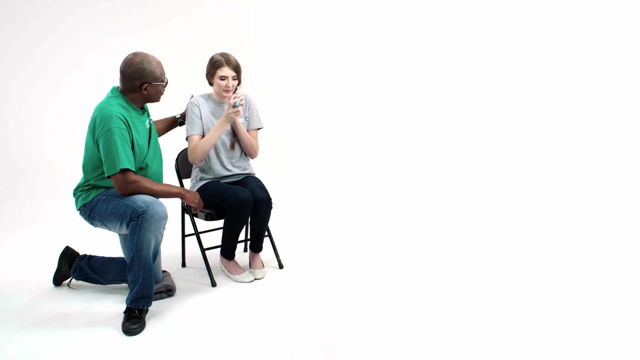 When treating someone having an asthma attack, keep calm, Reassure them and advise them to use their reliever inhaler straight away. Advise them to use a spacer, if they have one. Amy, use the spacer with the inhaler. Yes, Well done, Well done. Ask them to breathe. 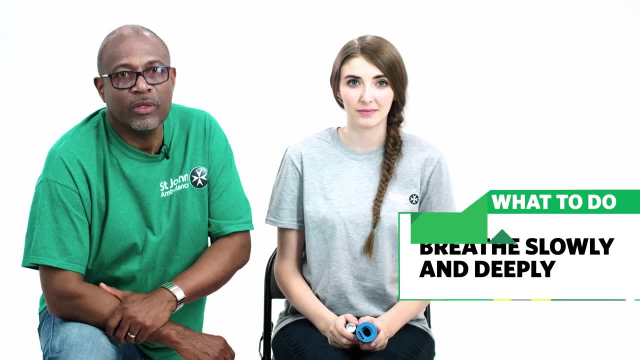 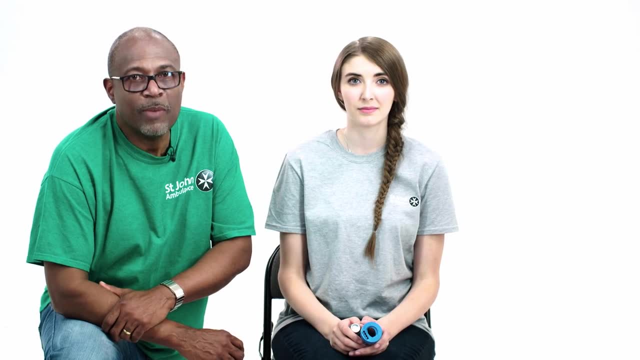 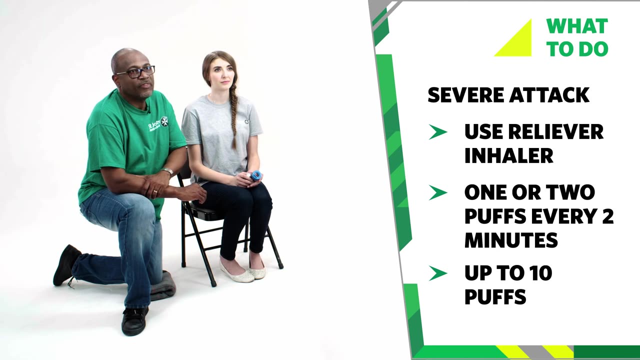 slowly and deeply To help control their breathing. sit them down in a comfortable position. If it doesn't get any better within a few minutes, it may be a severe attack. Get them to take one or two puffs of the inhaler every two minutes until they've had 10 puffs, If this is their 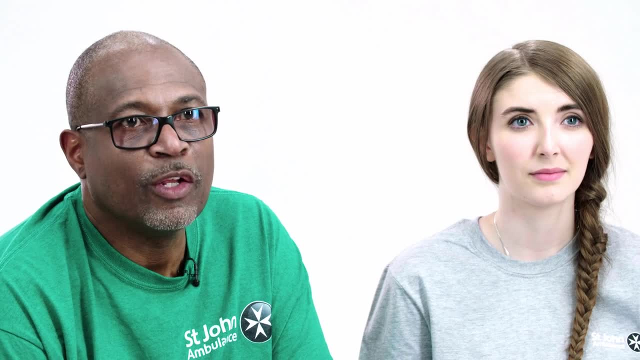 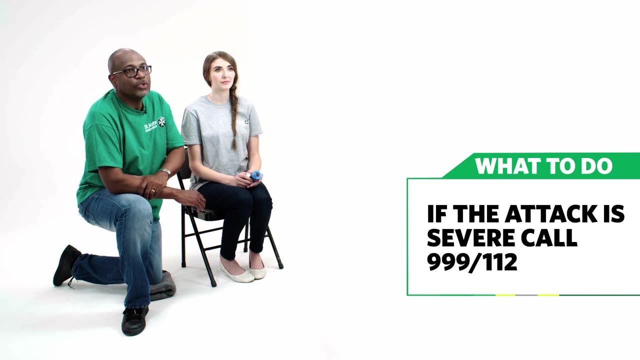 first attack. the attack is severe. they're not getting better, they're getting worse or they become exhausted. call 999 or 112 for emergency services. Thank you For emergency help. help them to continue to use the inhaler as needed. Keep checking. 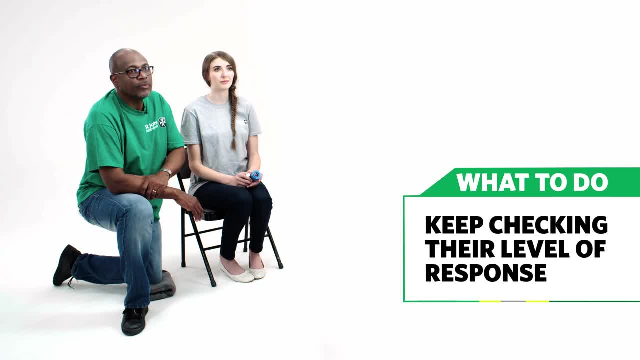 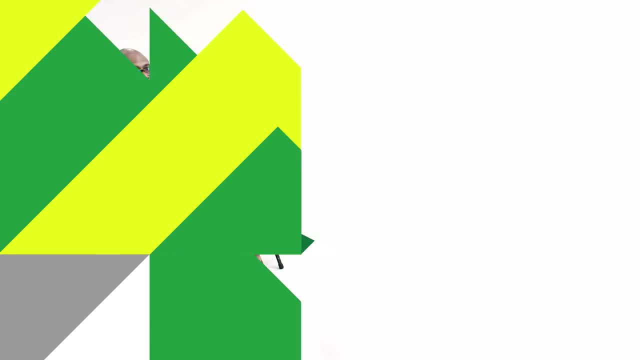 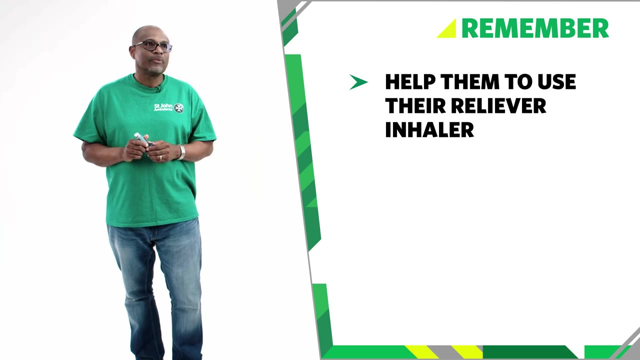 their breathing pulse and level of response If they do become unresponsive at any time. treat a casualty who is unresponsive, So remember, reassure them, Help them to use their reliever inhaler If the attack is severe. call 999 or 112 for emergency help and monitor their 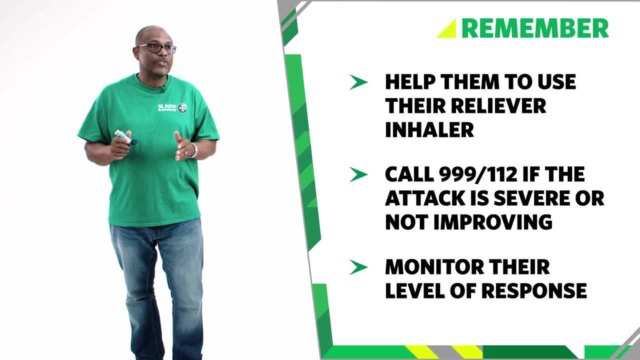 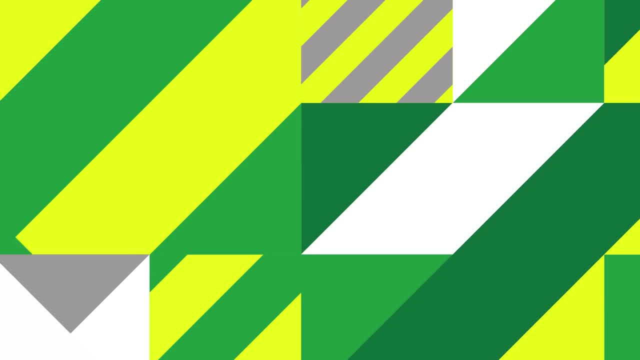 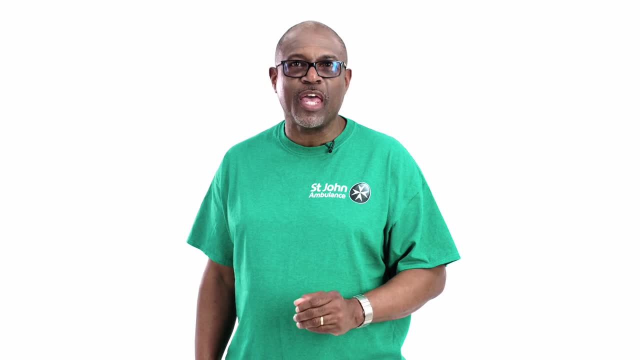 level of response. If they become unresponsive, treat as an unresponsive casualty, And that's how we help someone with an asthma attack. If this video has been helpful to you, help support St John Ambulance by going to sjaorguk forward slash donate. St John Ambulance.